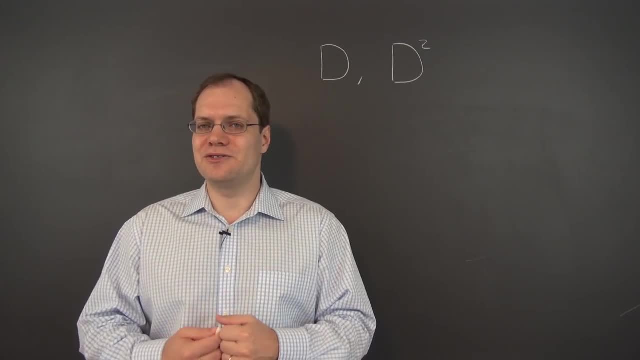 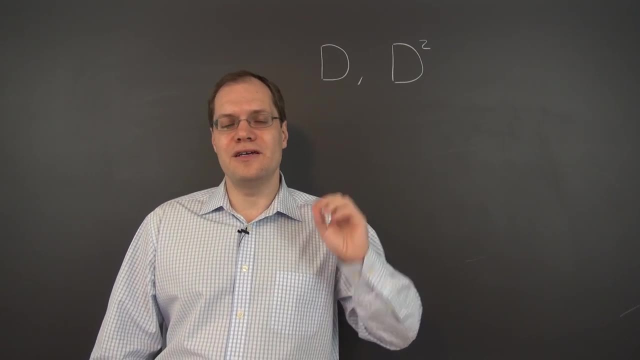 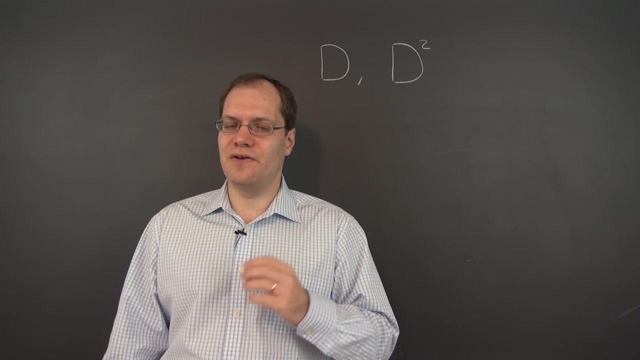 science of applying C, Similar ideas inspired by geometry, to all different kinds of objects. The questions we'll be asking are: are these operators linear? If they're linear, what are the eigenvalues and what are the eigenvectors? We're thinking of functions as vectors. Very appropriate. 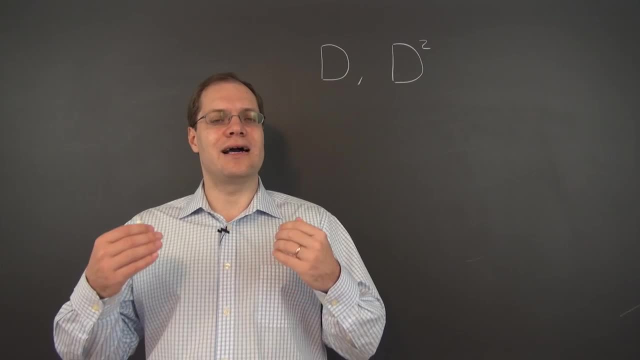 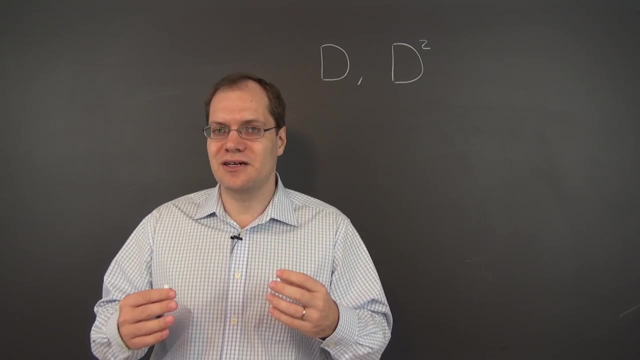 questions. One change in terminology: instead of calling them eigenvectors, we're going to call them eigenfunctions. But of course it's the same thing and maybe in the context of a linear algebra discussion it would be good to stick to eigenvectors. But that's just not the tradition. The tradition. 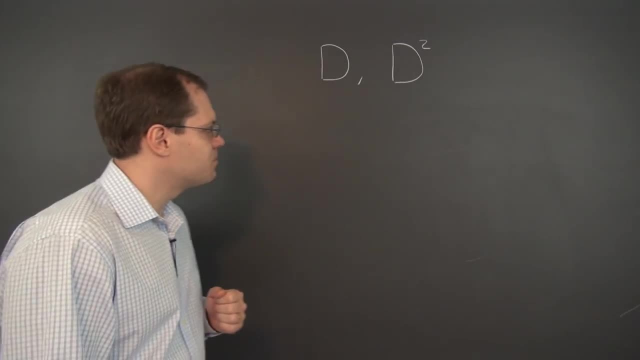 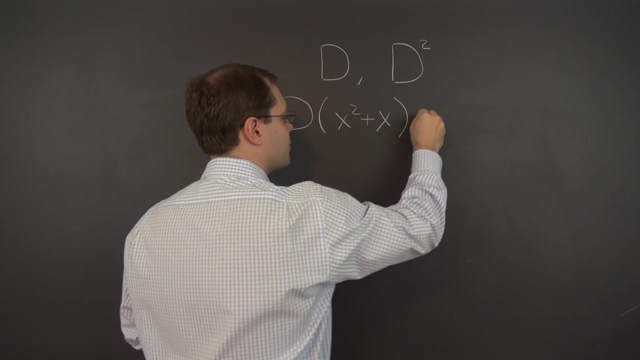 is to call them eigenfunctions, so we'll go along with that tradition. So just a couple examples. For example: d of x squared plus x equals…of course you know what it equals: It's the derivative of x squared plus x. See what a transformation. 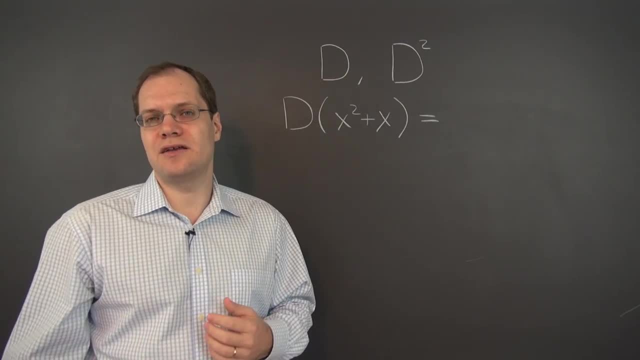 is. it's a mapping. The input is a function, the output is another function. There's a rule for converting the input function to the output function, for example, Theул of og and ofg, uor and ofg, ofg and ofg and ofg. it's also used for increasing the ont групп. 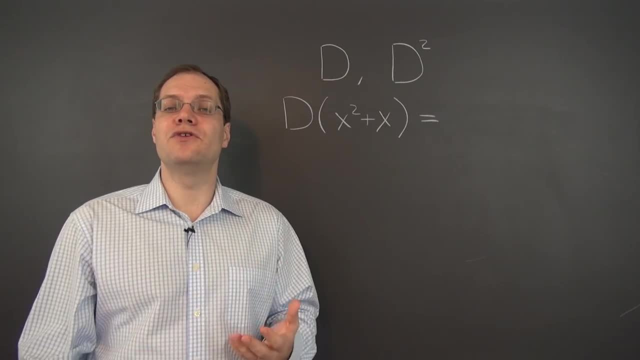 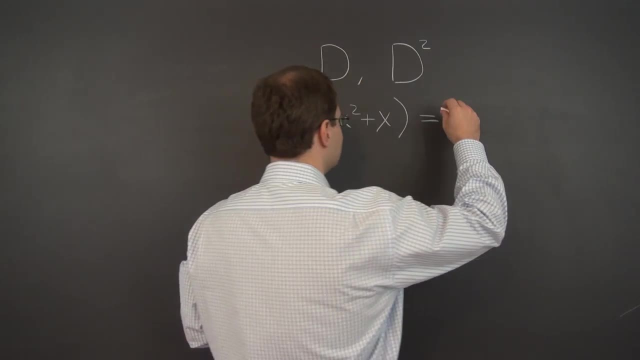 function to the output function, and it is up to me to give you that rule, and then, once the rule is given, we'll analyze it together. So, of course, the derivative of x squared plus x is 2x plus 1, and that's our first example. You 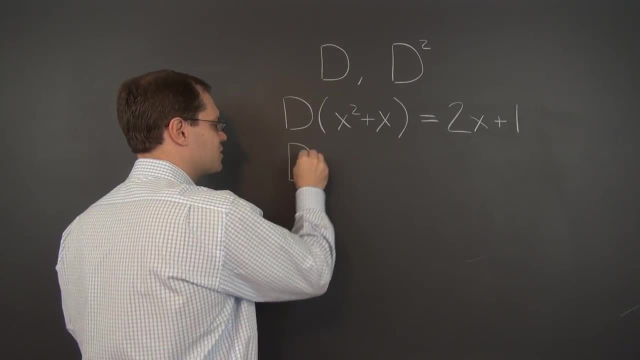 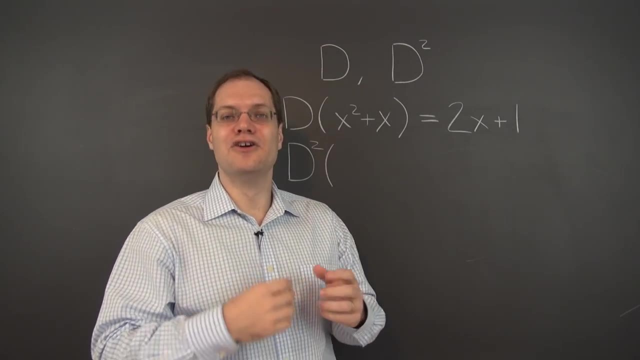 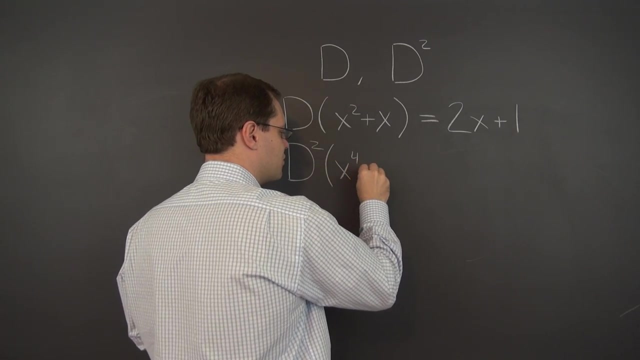 should probably consider a couple more. Well, how about we'll go straight for the second derivative. So here we're doing four things at once: Two different linear- we don't know yet that they're linear- Two different transformations, two different spaces. So let's stick to polynomials here: x to the fourth minus. 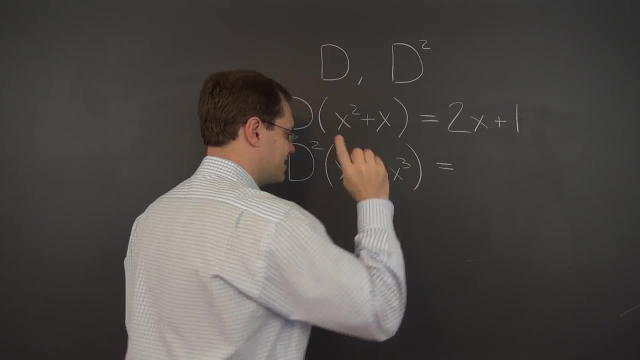 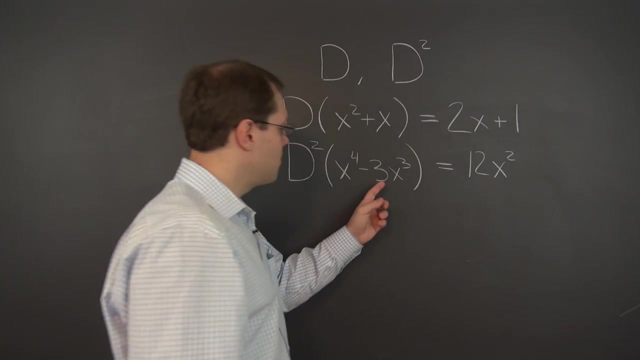 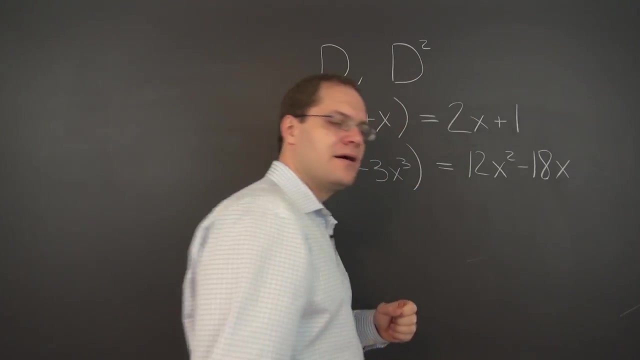 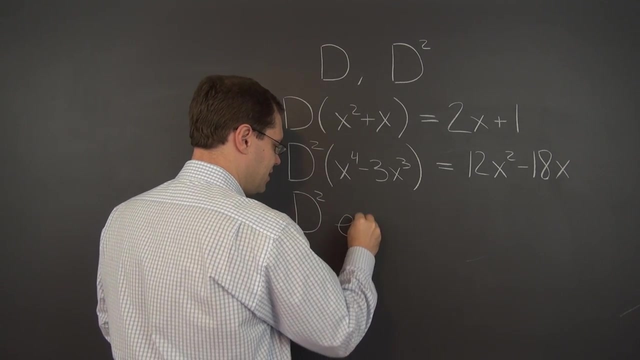 3x cubed and we're now taking the second derivative, so this becomes 12x squared, 12x squared minus 18x. How about an example with still the second derivative, but a function that's not a polynomial? How about e to the 2x? 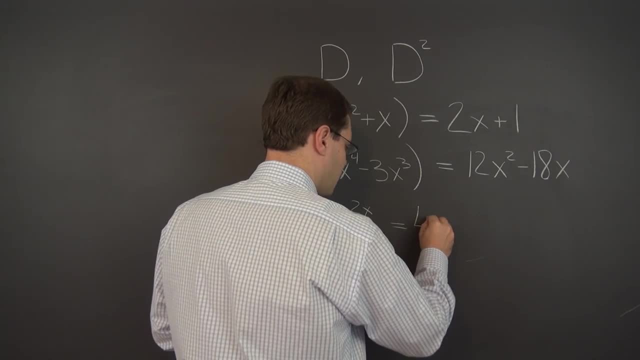 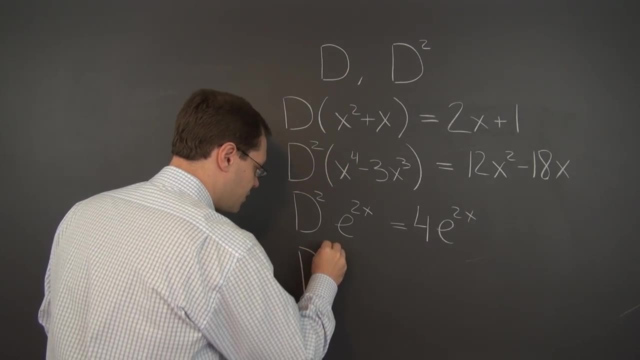 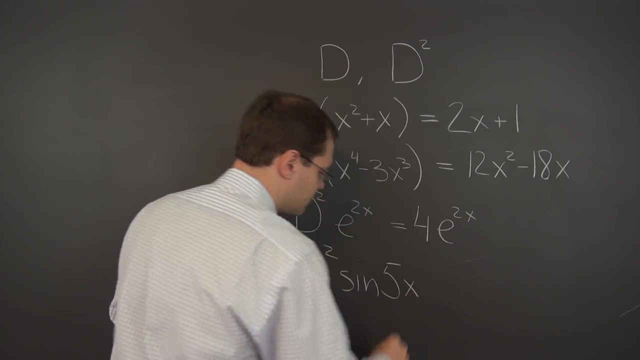 And of course the answer is 4 times e to the 2x. Let's throw in a sine. the derivative squared second derivative of sine of 5x equals minus 25.. Sine of 5x equals minus 25.. 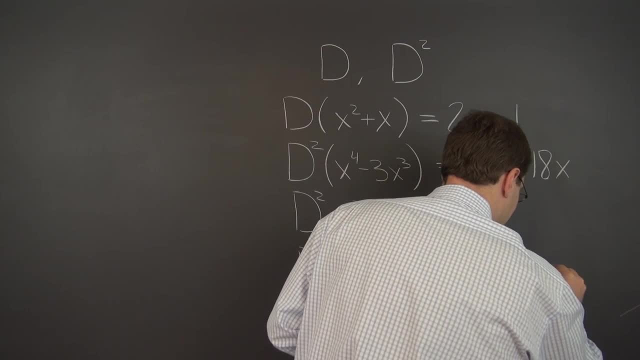 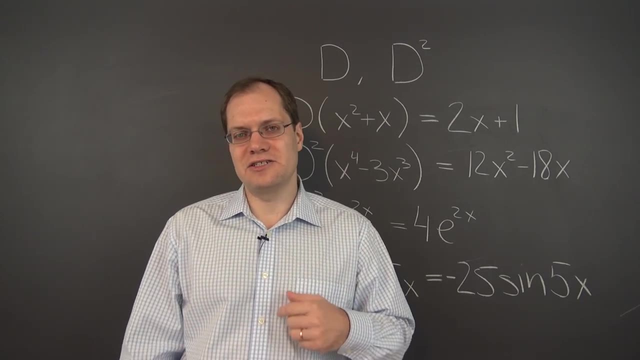 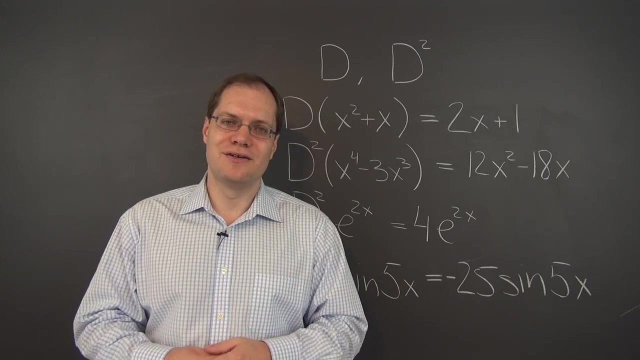 25 sine of 5x. And this is just about all the calculus you need to know for this discussion, Just being able to find these elementary derivatives. So we're not going back to calculus. This is not a course in calculus. There won't be any. 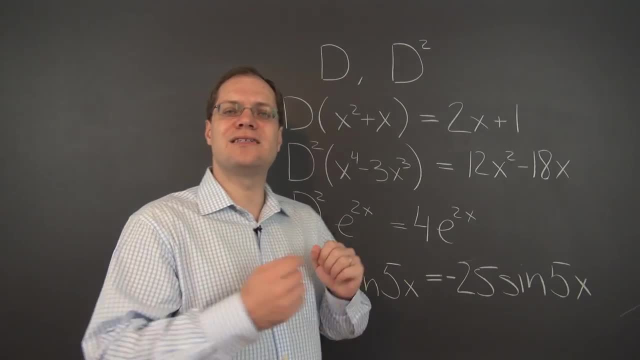 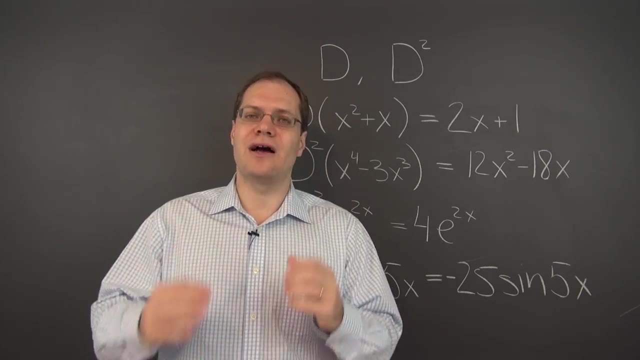 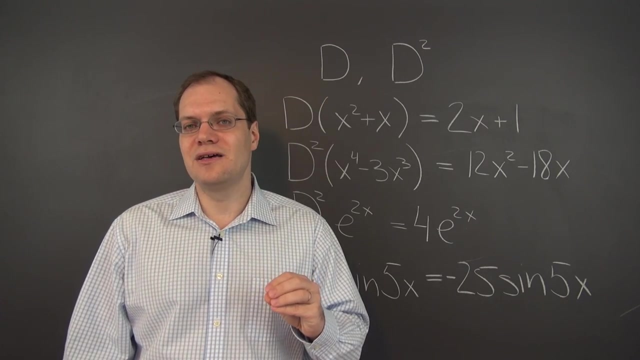 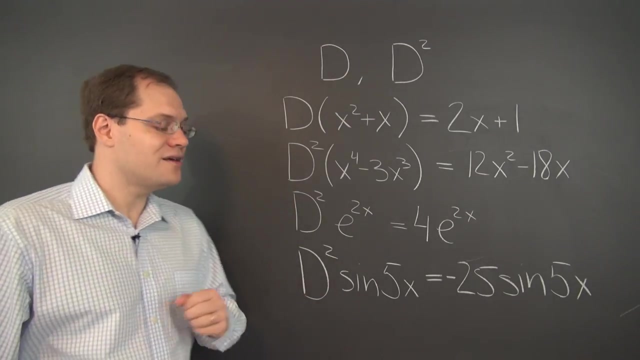 calculus review. of course, We're just extracting a part of calculus that has the linear algebra framework, or that can be described in linear algebra terms, and talking about derivatives as operators or transformations, and we will now determine whether or not they're linear is very much a subject in linear algebra. Okay, is this transformation linear or are 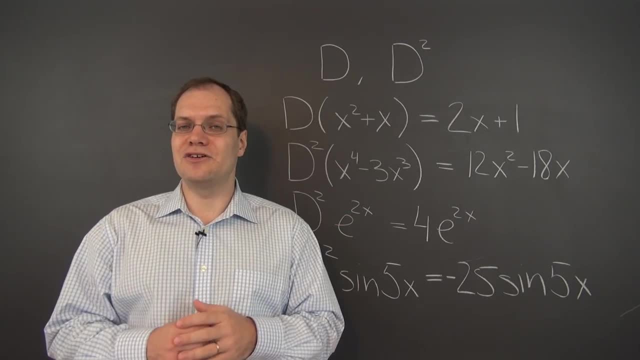 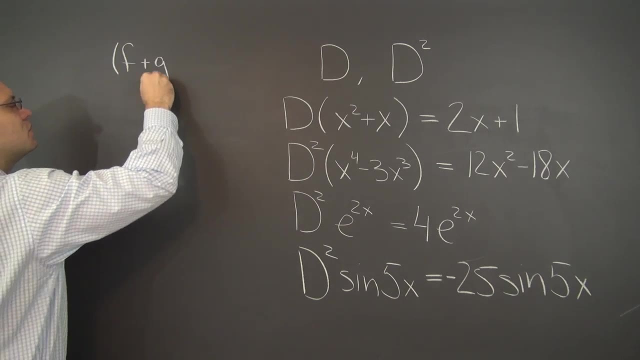 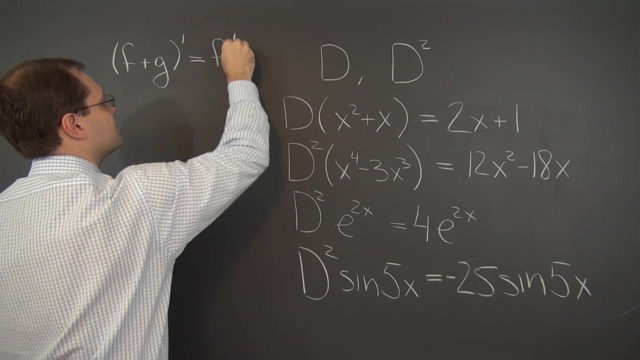 these transformations linear? And the answer is, of course. they are What you think of as some formulas in calculus. let me use the prime notation just so that it looks familiar. the derivative of the sum is, of course, the sum of the derivatives. You usually use this rule without giving it much thought. 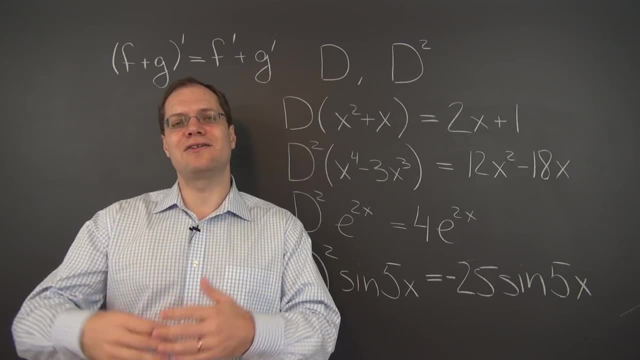 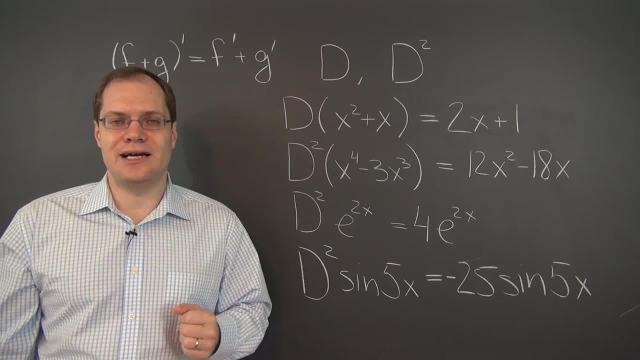 and you shouldn't. it's completely trivial, it's fundamental. calculus wouldn't exist as we know it if this rule wasn't there. but from our point of view it means that we're halfway to linearity. It means that the derivative operator- and of course the same would go for the second derivative, doesn't matter. 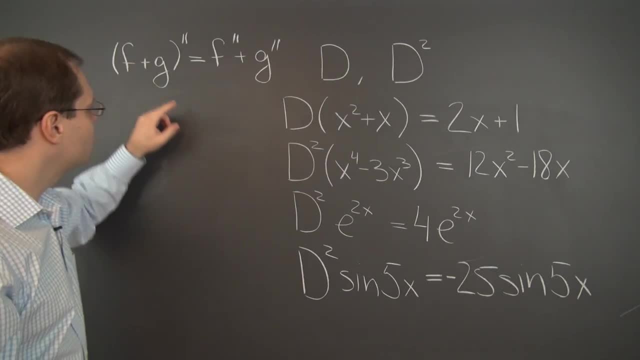 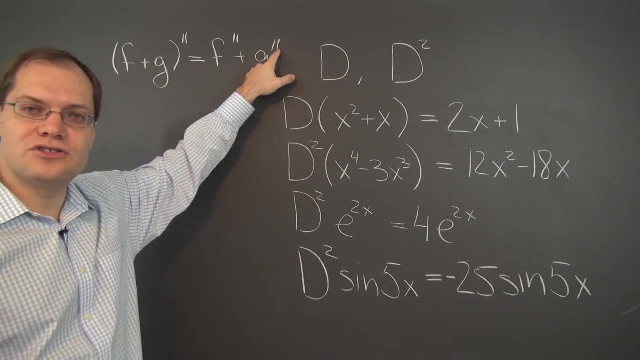 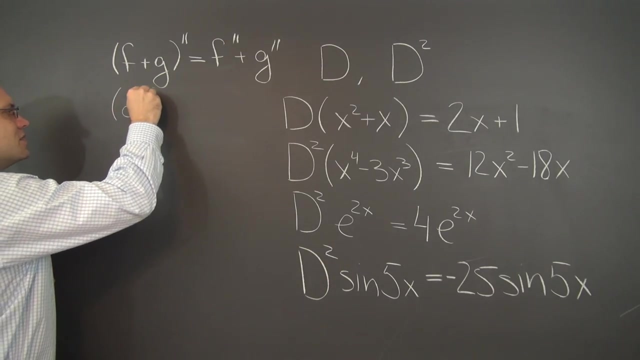 is the sort of operator for which it doesn't matter whether you add the two vectors first and then transform the result, or whether you transform the individual vectors and then add together the results. So that's half of linearity, and the other half, of course, comes from this product rule. This 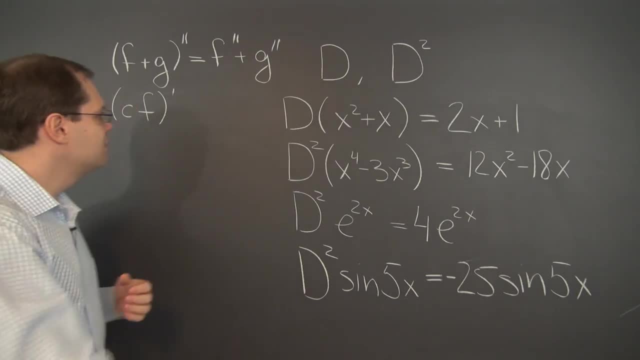 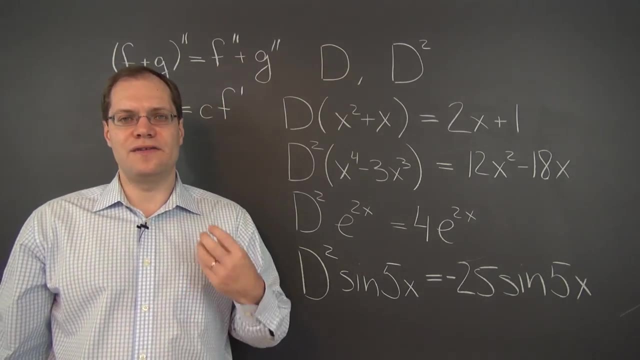 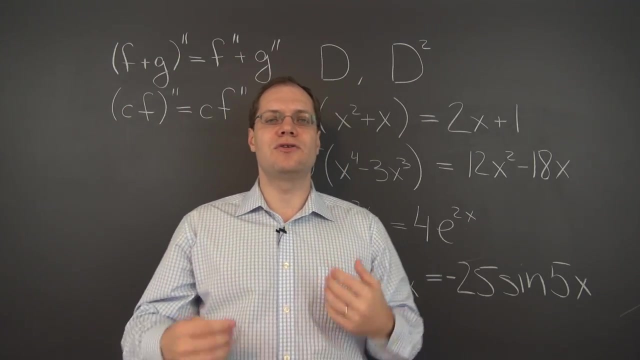 is not product rule. this is multiplication by a scalar rule and maybe it's a special set of the product rule, but it reads like this: and that's the second half of linearity works just as well for the second derivative. So we have both of these rules for first and second derivative. So, yes, this. 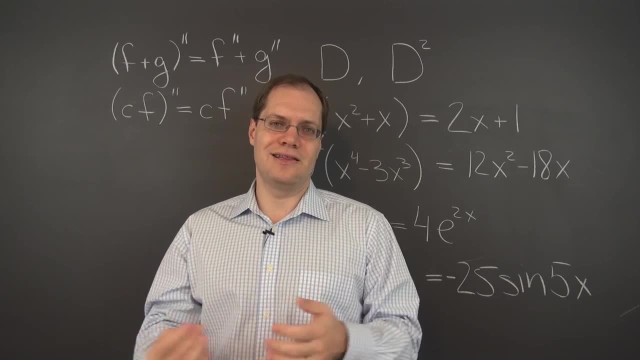 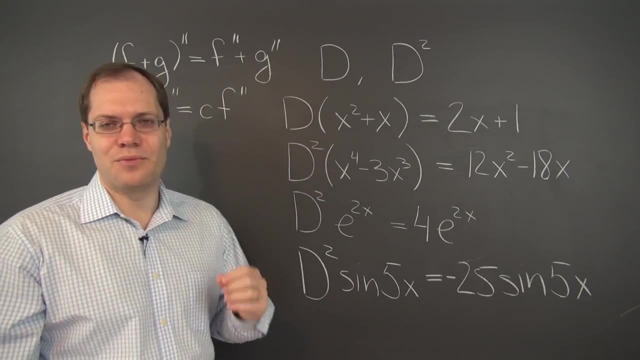 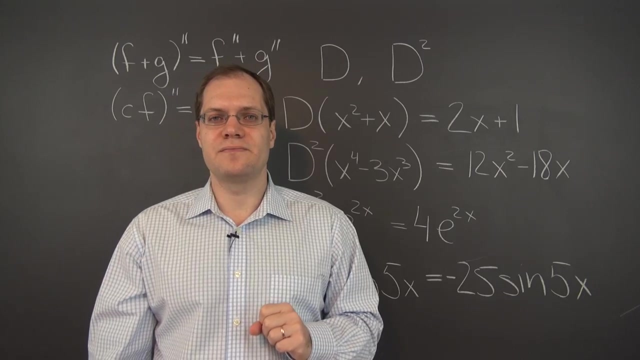 transformation. these transformations are linear and once we have a linear transformation, what's the next obvious question, natural question, important question is: what are the eigenvalues, and in this case, eigenfunctions, of these two transformations? So let's try to answer these questions by trial and error. First, 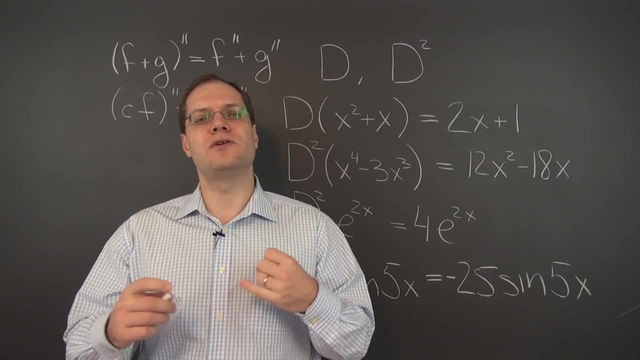 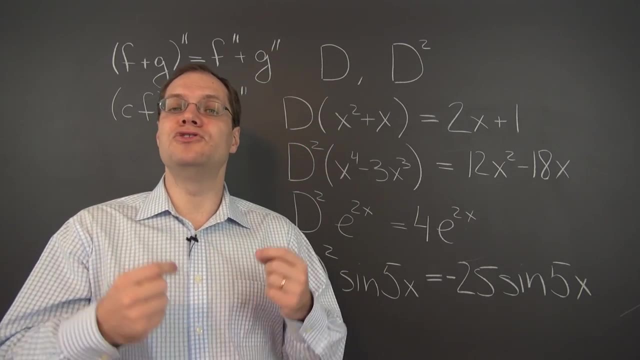 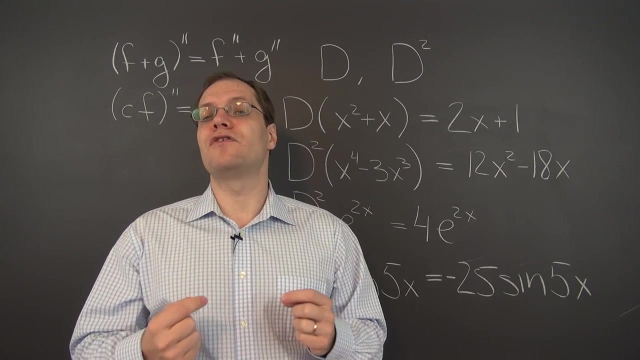 let's stick to the space of polynomials And then we'll talk about functions in general. Can you think of a polynomial that becomes a multiple, whose derivative and then second derivative is a multiple of the original polynomial? At your first thought, maybe. well, there's no such. 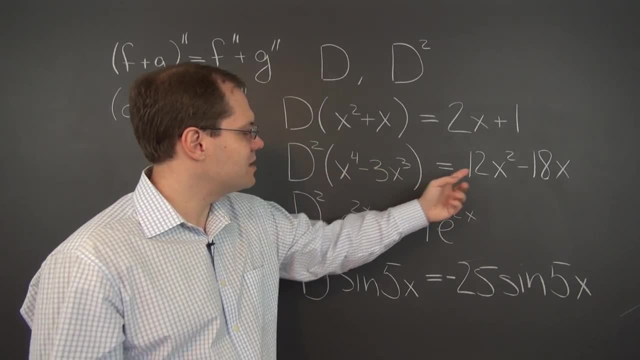 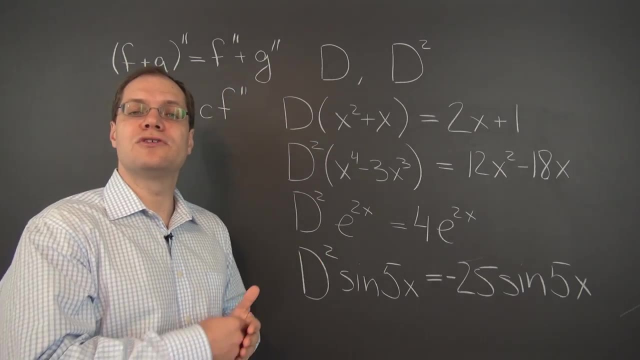 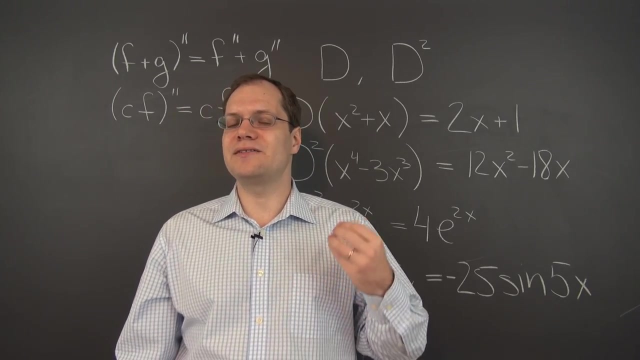 polynomial, because anything with x to the fourth will end up with something less than x to the fourth, because the derivative knocks the power down. So how can the result be a multiple of the original polynomial Of the pre-image if it has a different power? That's a very correct way of. 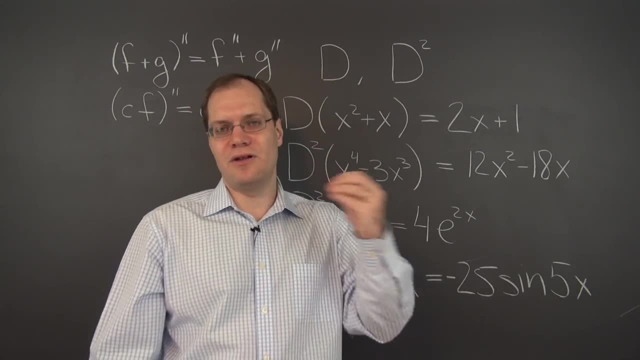 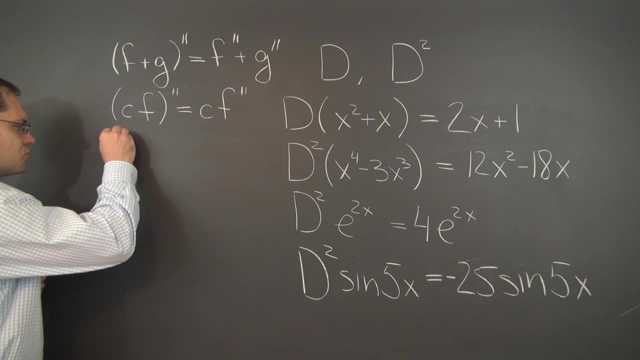 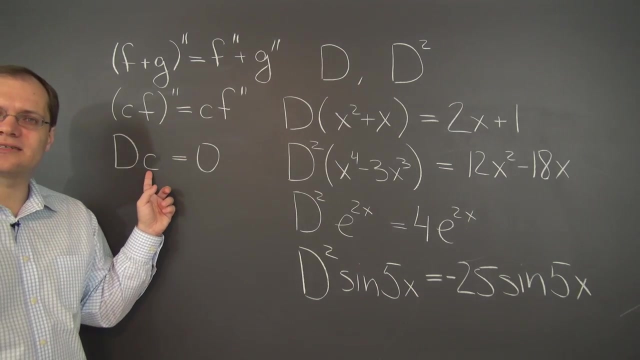 reasoning. It typically won't be a multiple of what you started out with, But there is one little exception, and that's the constant function. The derivative of a constant function is zero, So this is constant the function, not constant the number. Let me draw a graph of this function As any function. 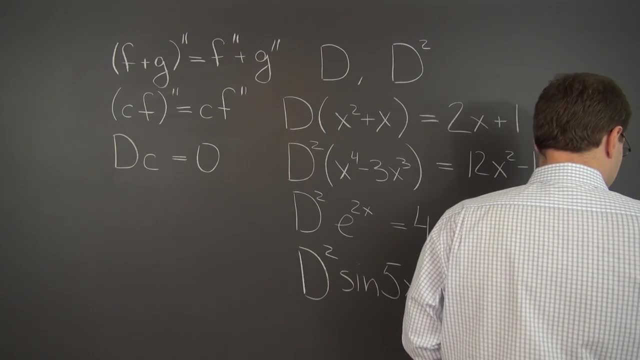 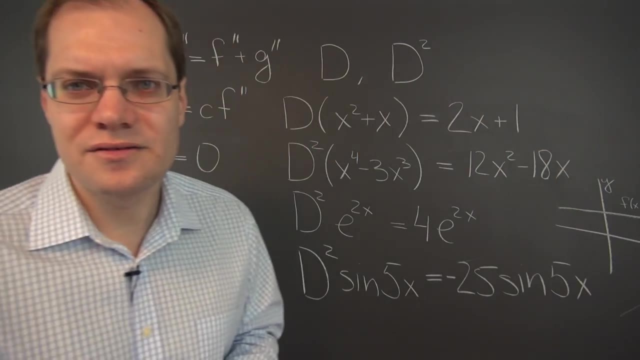 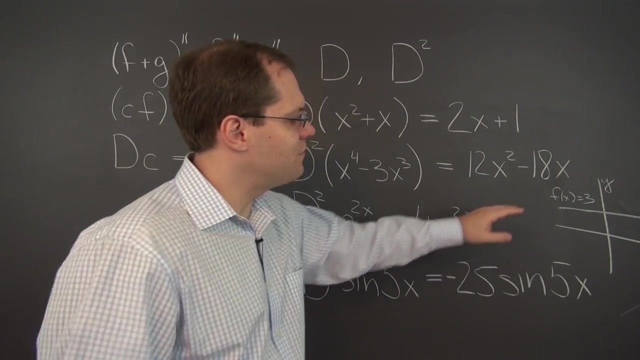 it has a graph, and if c equals 3, then maybe that's the graph. Alright, this has f of x. Is it even in the shot? Barely, but you know what I mean. f of x equals 3.. There you go. A function like that, a constant function, its. 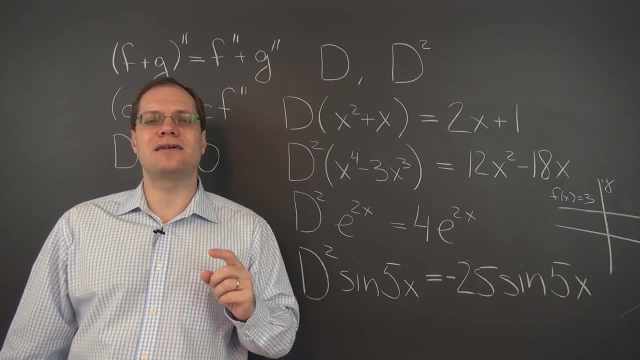 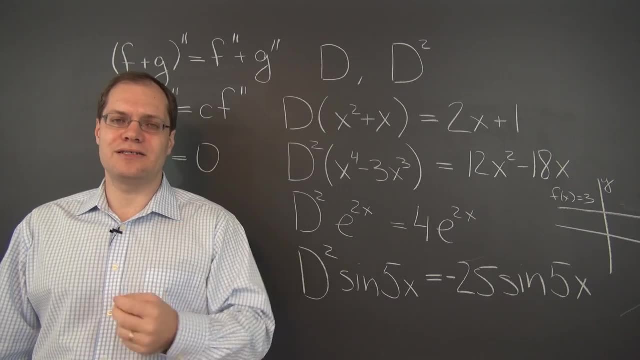 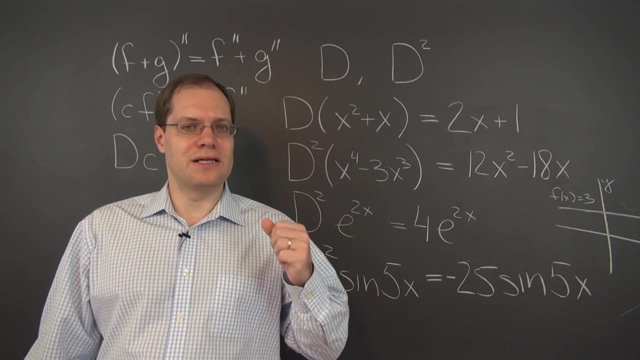 derivative is zero. And this is our second example of an eigenfunction eigenvector. you may think of it as eigenfunction with the zero corresponding eigenvalue. So an eigenvector cannot be zero. I'm interesting- inapplicable, But a eigenvector eigenvalue may very much, much. 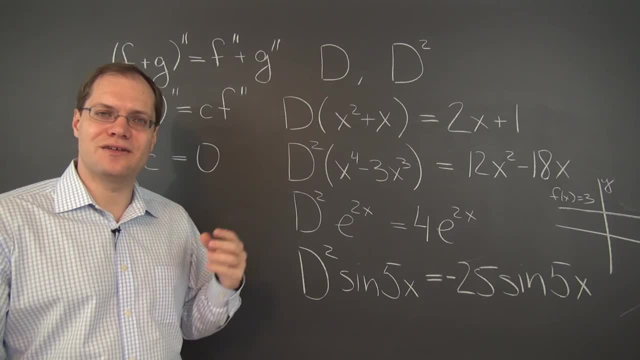 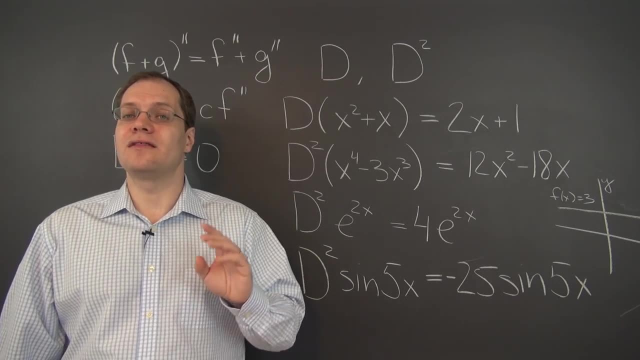 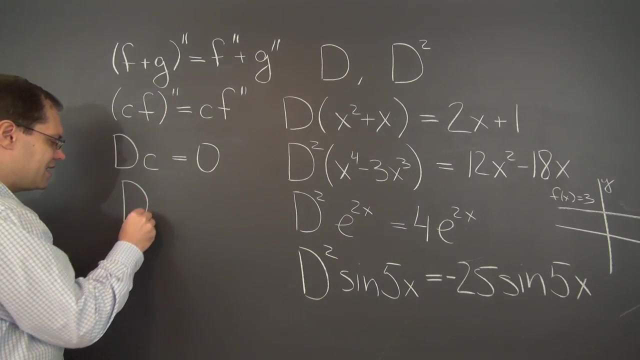 be zero, And here it's actually one of the more interesting eigenvalues. And here we're definitely seeing another example of the zero eigenvalue. That's that's it for the first derivative. Of course, for the second derivative, this eigenspace is a little bit richer because you can take any linear function. 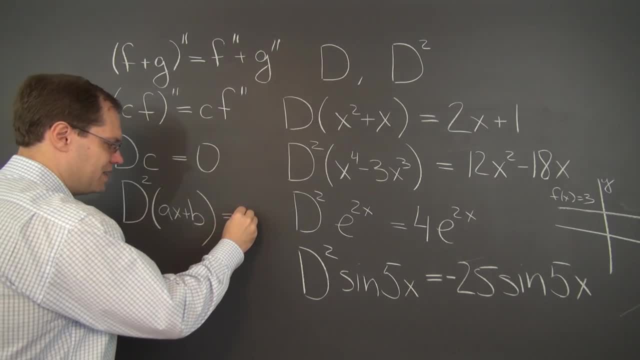 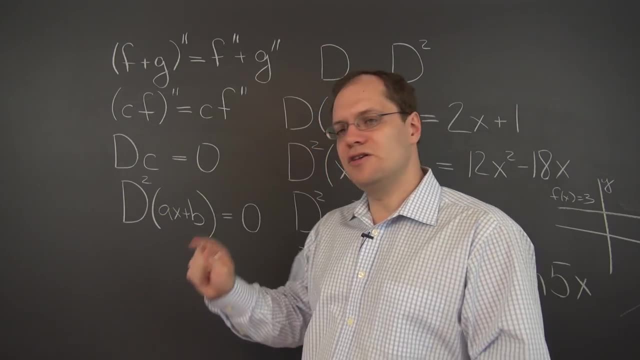 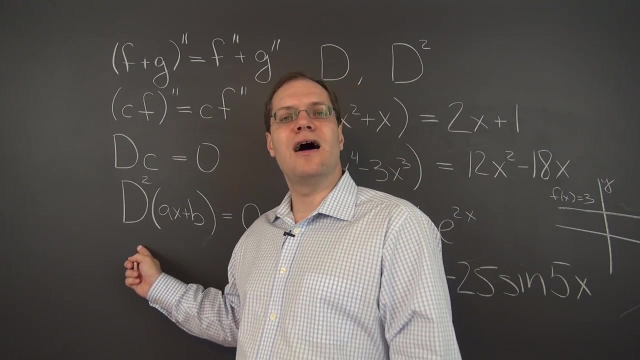 any linear function ends up being zero. So this eigenspace corresponding to the eigenvalue zero is two-dimensional. This was one-dimensional and in the case of the second derivative, the eigenspace corresponding to the eigenvalue of zero. 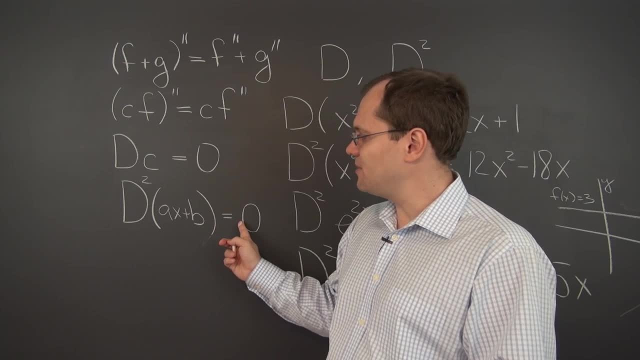 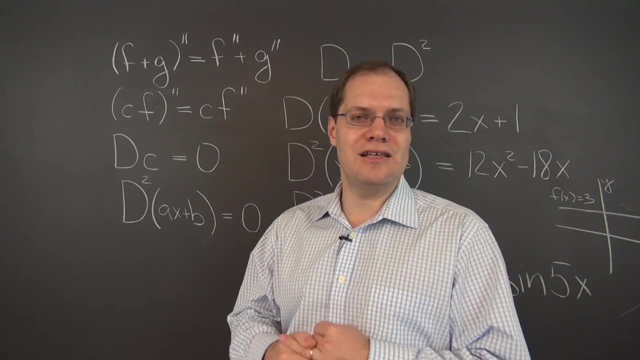 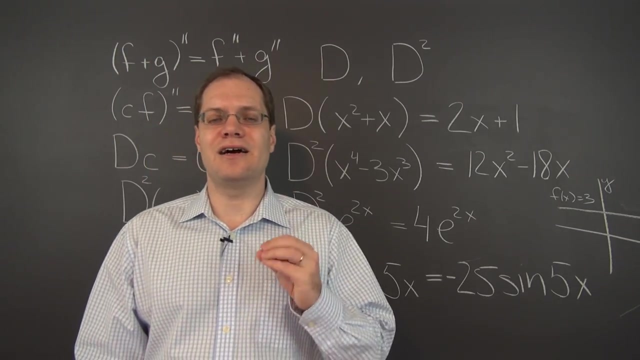 is richer, It is two-dimensional. The third derivative would have a three-dimensional eigenspace corresponding to the eigenvalue zero, and so forth. Very interesting, But that's it for polynomials. Polynomials don't have any other eigenfunctions because that logic of the derivative knocking down. 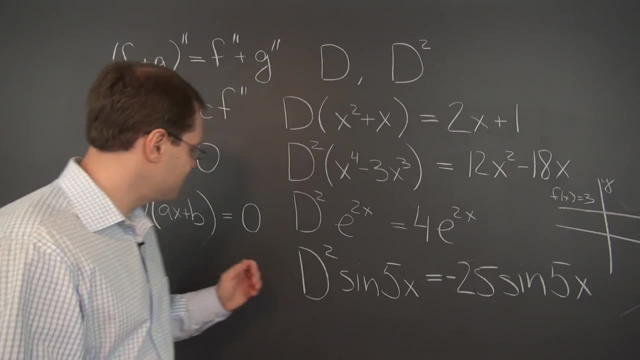 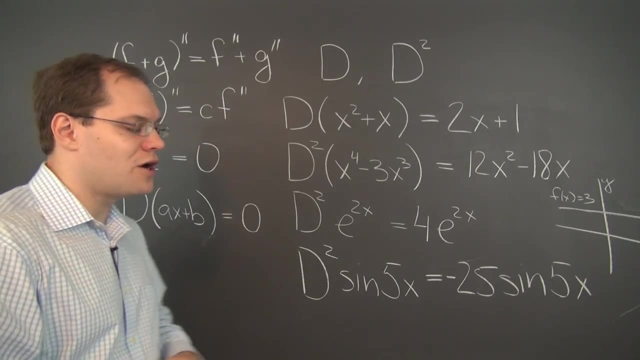 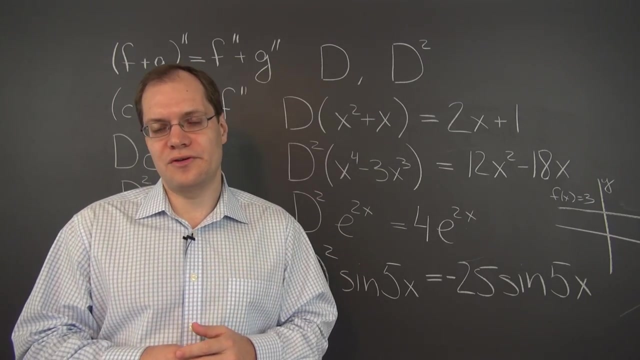 the power is the correct logic. It's just that sometimes you end up with zero. That's the only exception. It fits well within that logic. Now, what if we now broaden our view to general functions? What are the eigenfunctions of the derivative and the second derivative transformations when? 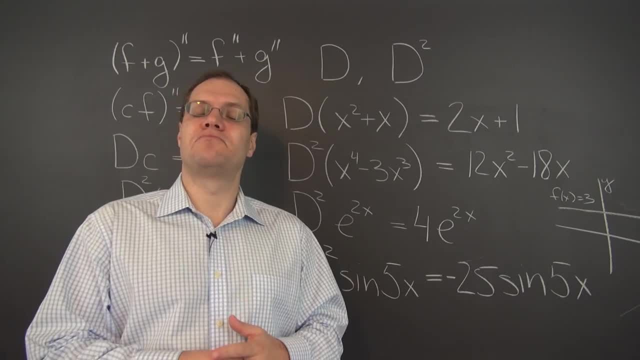 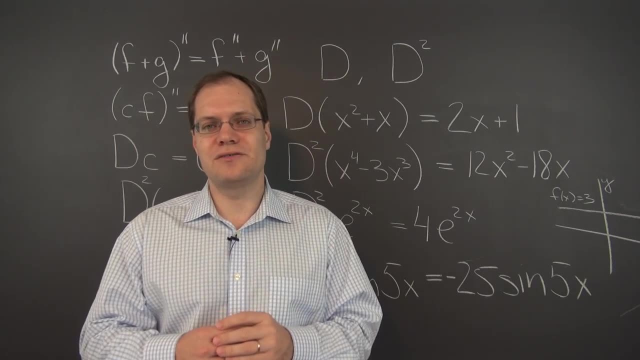 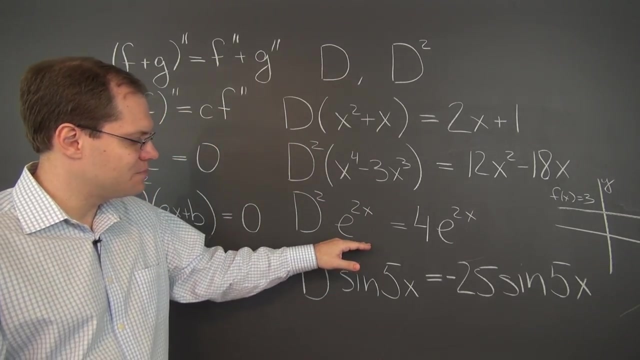 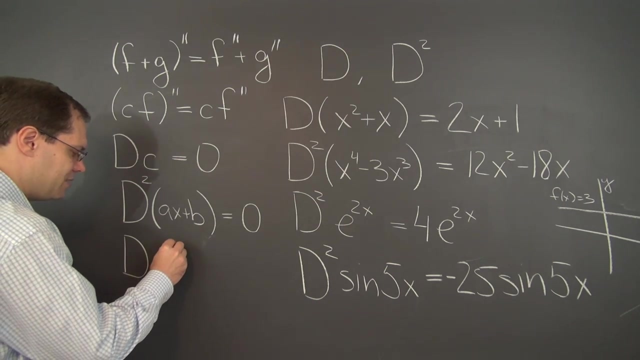 we allow all functions. Well, that makes of course these still apply, because polynomials are still general functions. But there is now a richer space of eigenfunctions, And actually there are some hints here. first, derivative: we can take e to any power, e to the. what would be a good 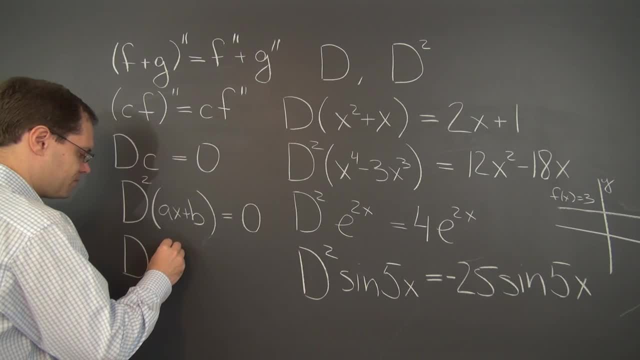 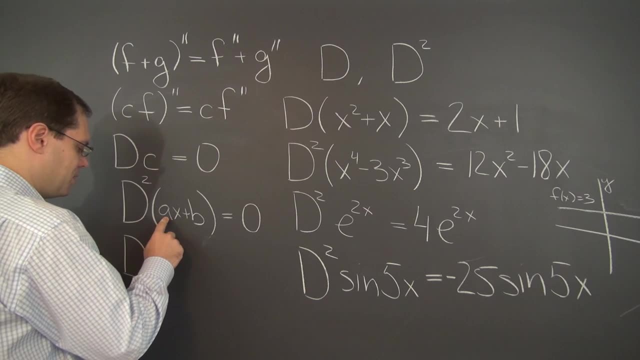 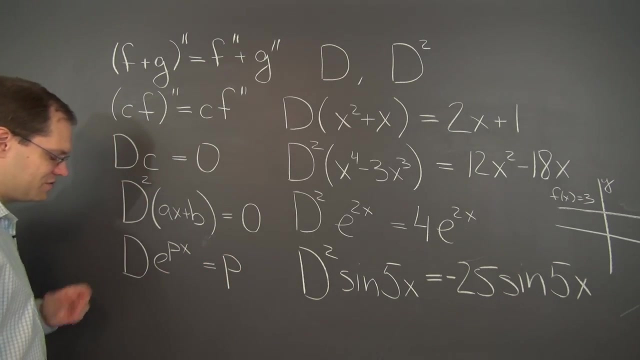 power letter for the power, let's call it. I don't want to use the letter a because a is used right here. let's use P for power. e to the P. X, where P is a constant is, of course, by the celebrated derivative chain rule and the celebrated 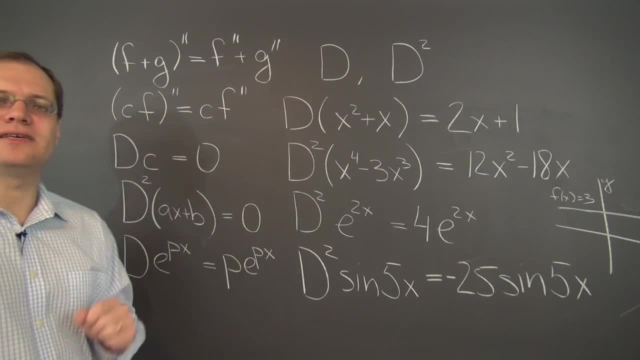 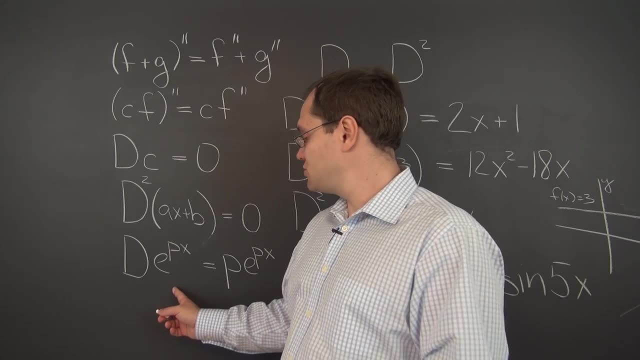 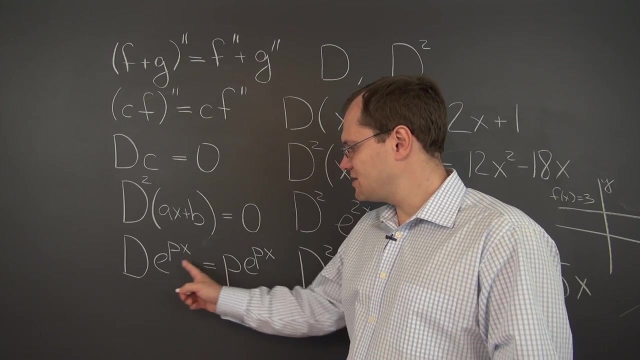 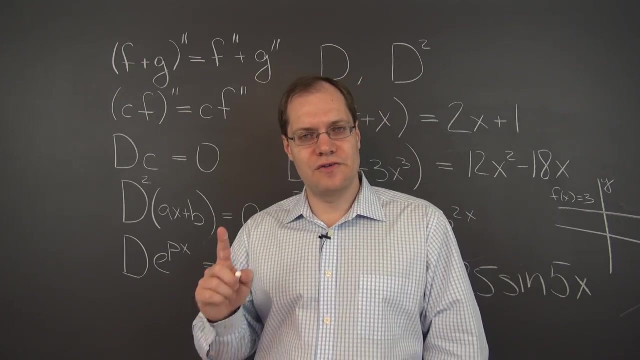 function in the differentiation table. P times e to the P X. now once again very familiar from calculus, but now you have a- much don't want to compare- a very interesting linear algebra perspective. this identity states that e to the P X, where P is any number, is an eigen function of the derivative operator with 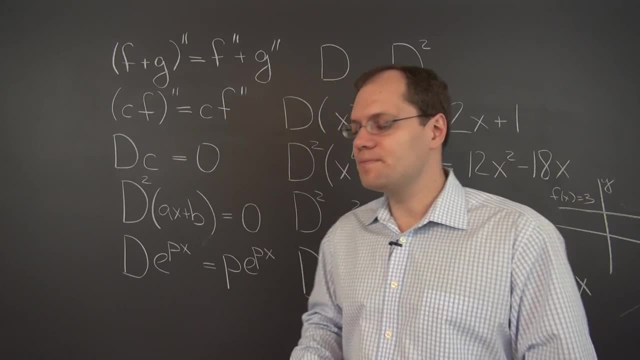 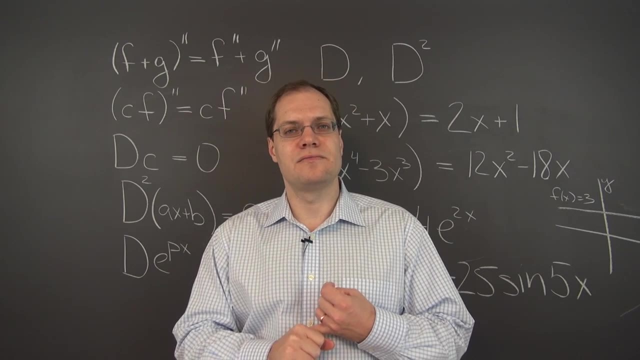 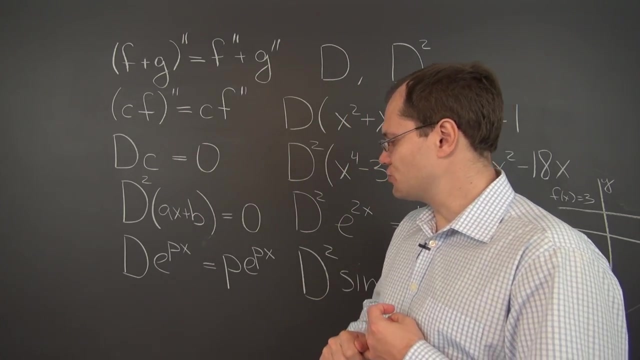 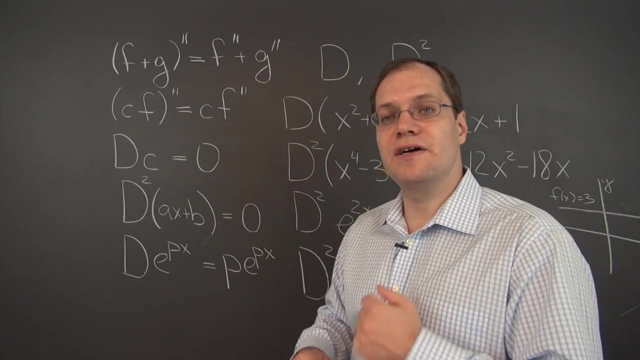 B with P bearing the corresponding eigenvalue. you and as you can see, this is our first example where there are infinitely many eigenvalues. there are infinitely many eigenvalues. any number is an eigenvalue of the derivative transformation- and we have infinitely many completely linearly independent eigen functions. very interesting example, something that's. 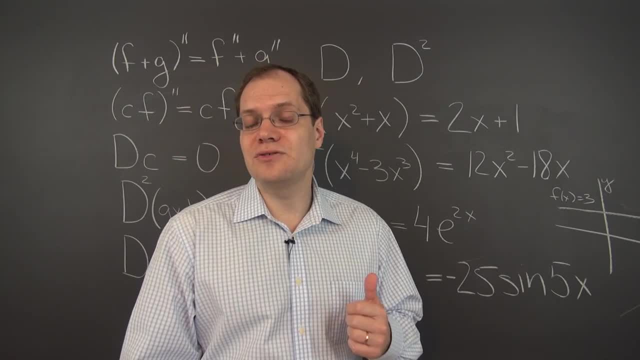 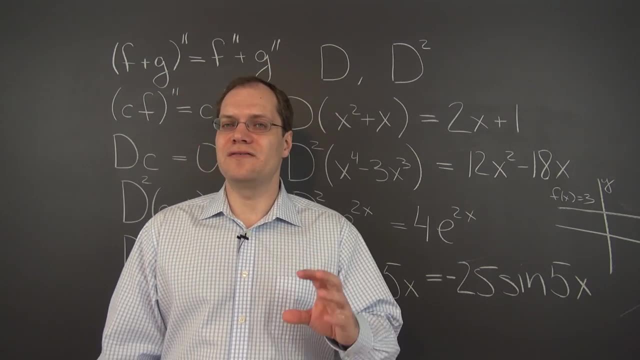 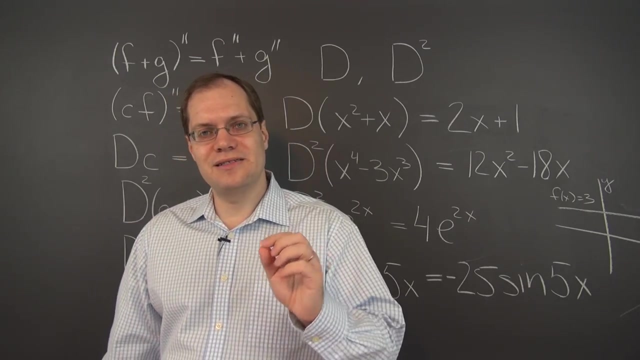 very good to keep in mind. and that's actually it for the space of functions. you are a function that is able to drive a particular function whenever you do not work a different function. if it isn't working, we could say that it is working. if this is a function, arizon, we can. hence it can't work with other functions. 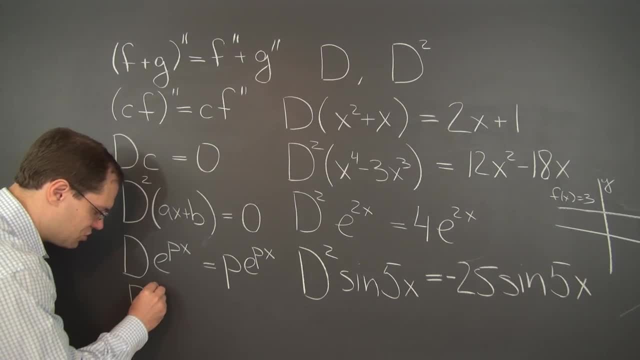 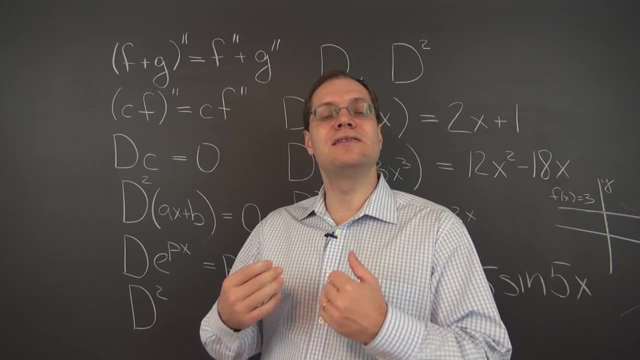 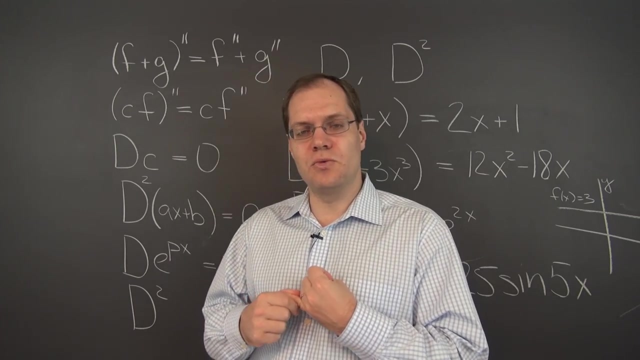 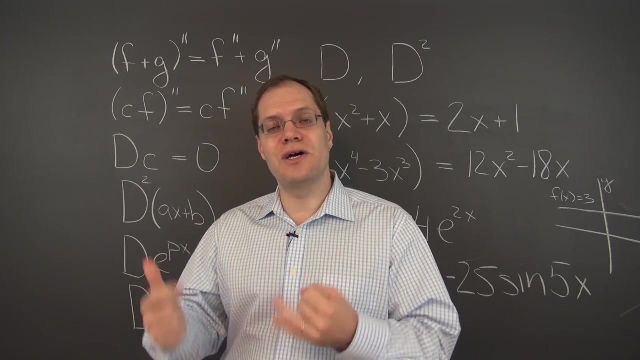 found together, so it is a function that is applicable to one another. Legislation: penser Grammar inherit from the primitive precisa. latte semaines significa a, wenn es bei der produces a multiple times the same thing and then, applying it again, multiplies that multiple squares the multiple. 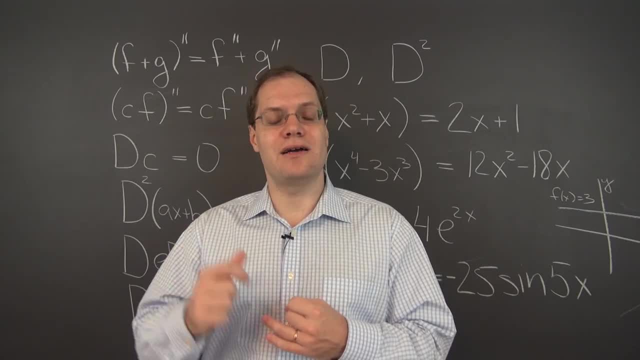 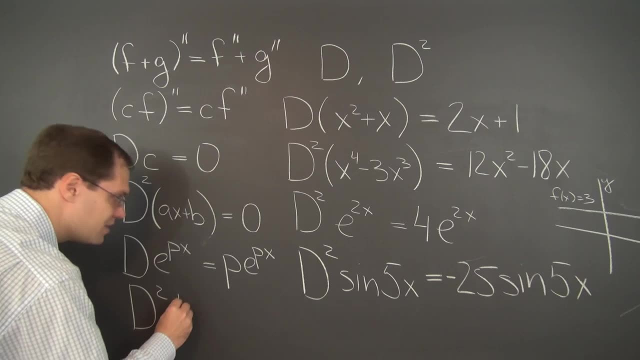 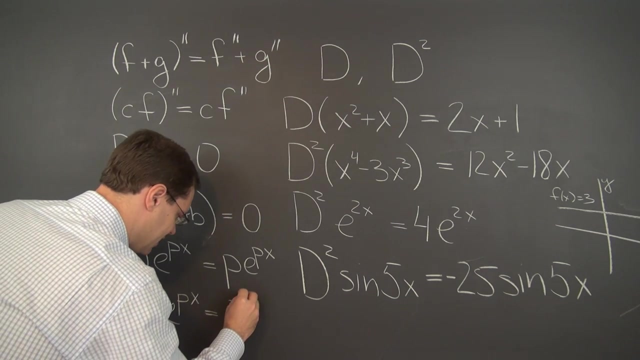 and once again produces the same thing. So it's that multiple squared times the same thing. So e to the px is still very much, and that's what you're seeing here. e to the px is very much still an eigenvector. 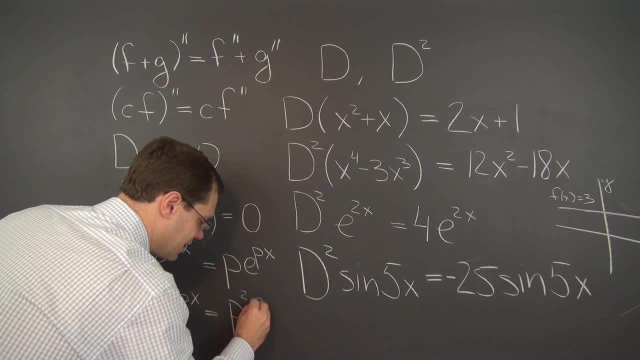 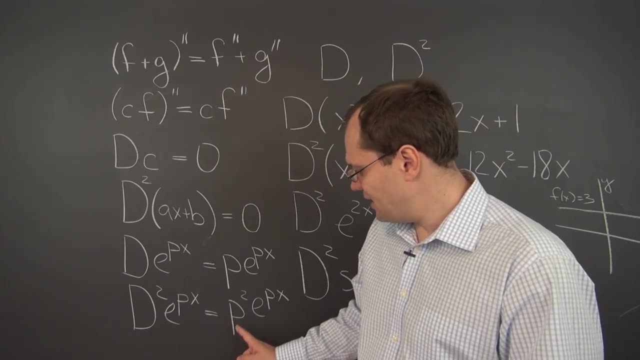 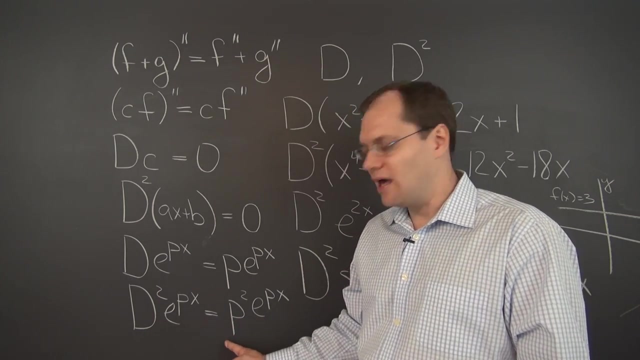 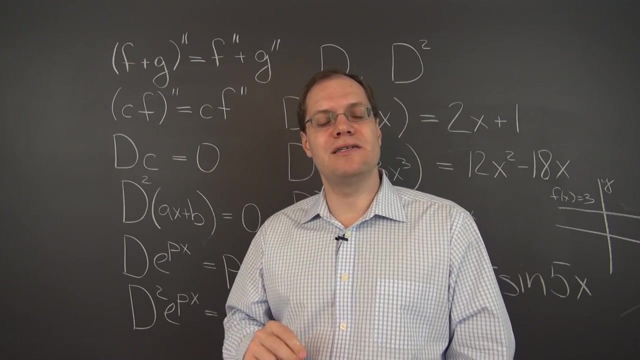 eigenfunction and the corresponding eigenvalue is p squared. Very interesting. So once again still infinitely many eigenvalues. but now this only gives us positive numbers, And to every positive value, such as 25, there are two corresponding eigenfunctions. 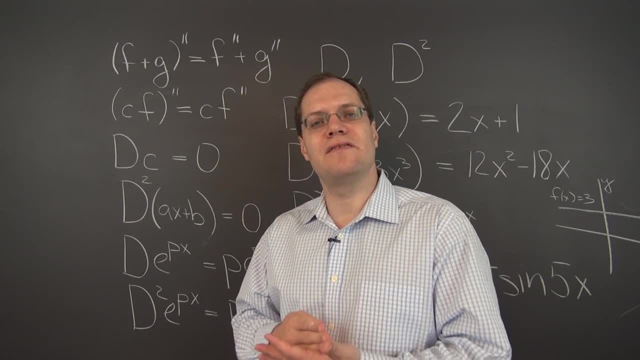 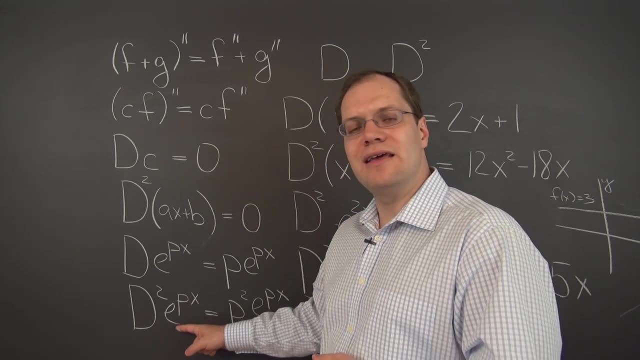 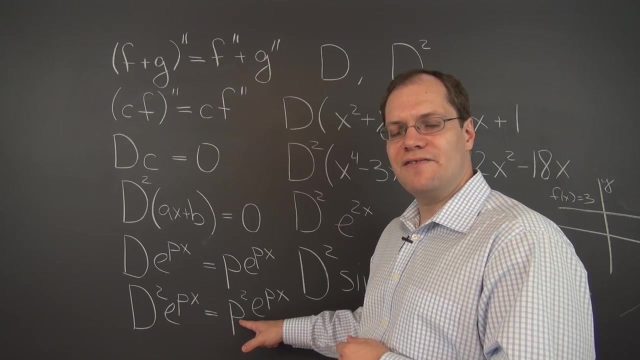 So the eigenspace corresponding to that eigenvector, the corresponding eigenvalue, is two-dimensional. It's e to the 5x and e to the minus 5x. Both will produce the same eigenvalue of 25.. So very interesting. 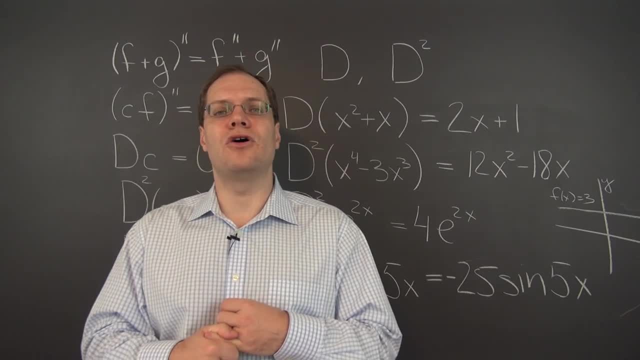 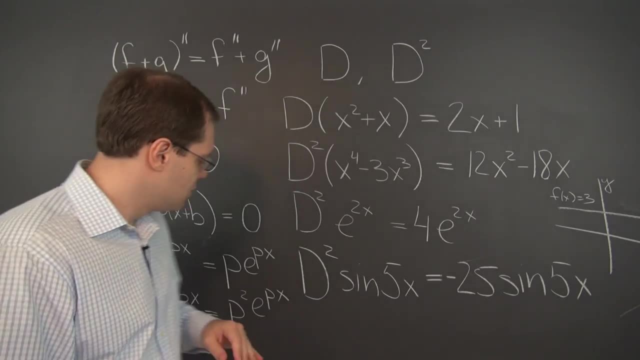 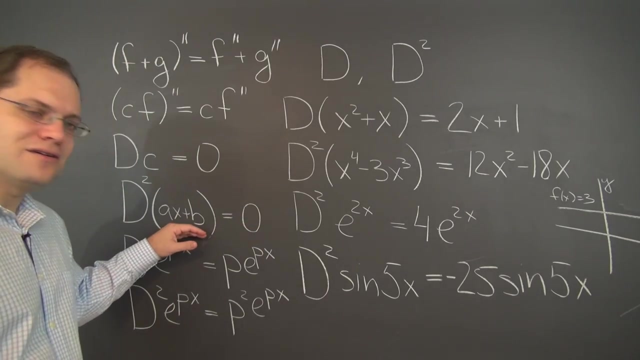 Still infinitely many eigenvalues, but now they're only positive numbers and the corresponding eigenspaces are two-dimensional, Whereas in this case the corresponding eigenspaces were one-dimensional. Very interesting, Kind of similar to this: Preserved the eigenvalue. 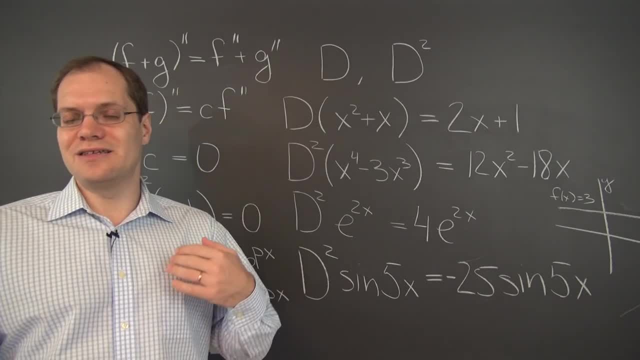 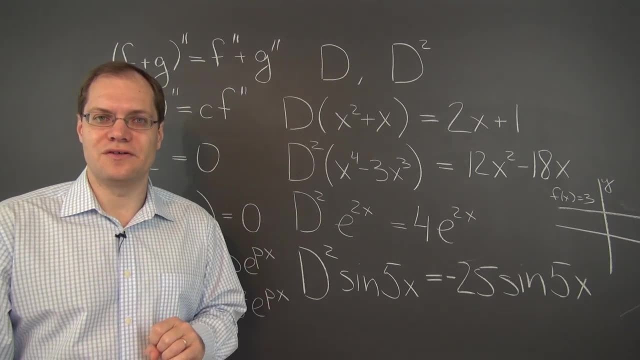 but now the eigenspace is two-dimensional. It seems like the dimensionality of all the eigenspaces corresponds to the order of the derivative. All right, but of course there is one more, and you can kind of see the clue right here. 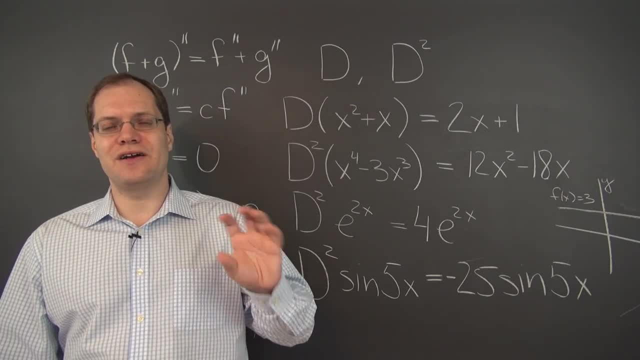 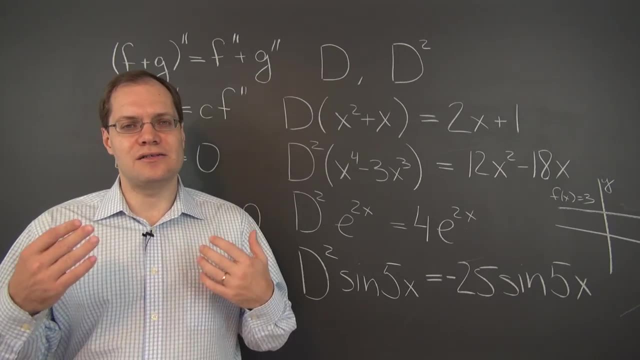 Well, maybe two more sines and cosines. We would have to think very carefully about the dimensionality of the corresponding eigenspaces, because sines and cosines mix in a very nice way according to the trigonometric formulas.